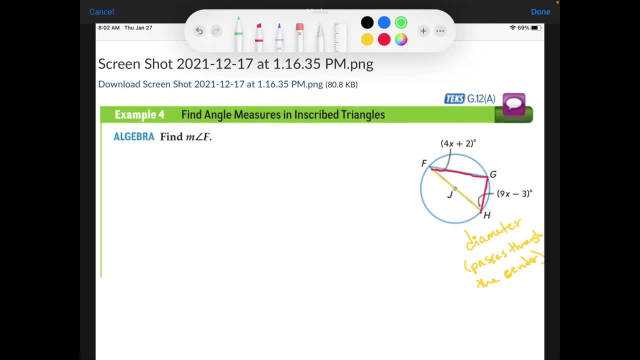 we can say that this angle, FGH, is creating a right triangle, which means that this angle right here is a 90 degree angle. Now that we know that, if we need to, we could kind of draw this out, draw the triangle outside of the circle. 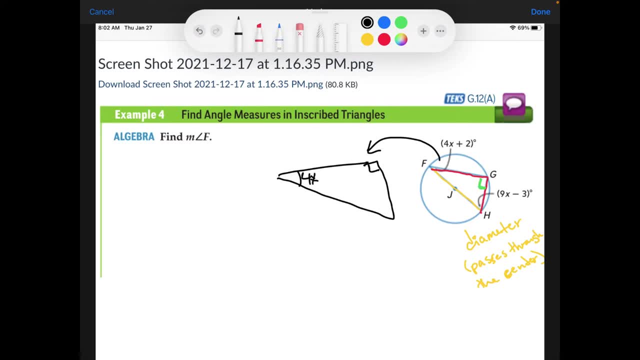 so we can recognize this kind of problem. We've done it before. This angle is 4X plus 2, and this angle is 9X minus 3.. Remember that the sum total of all the angles in a triangle equals 180.. So we're going to set everything equal to 180 and add up all these angles. So 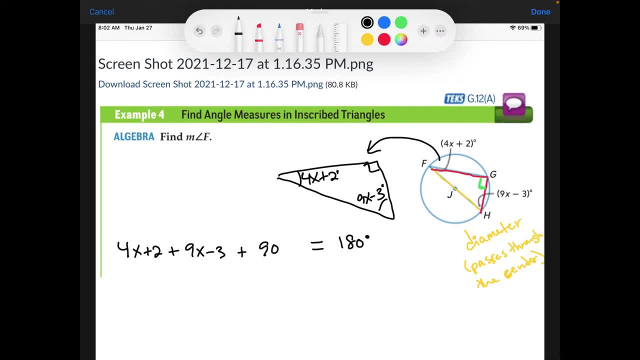 we're going to say 4X plus 2 plus 9X minus 3, and let's not forget the box. The square box is 90 degrees. So now that we have it set up, we can put this into Desmos. If we were going to solve this by, 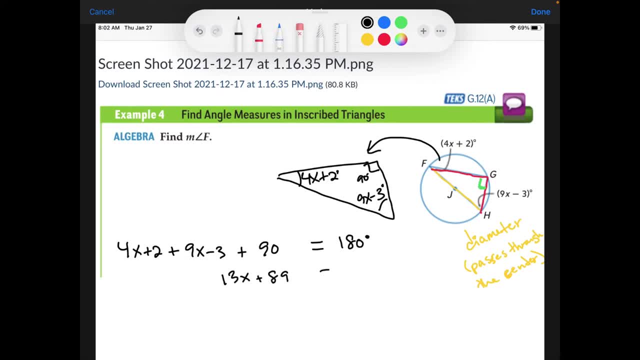 hand, we would end up with: 13X plus 89 equals 180 degrees. We could subtract 89 from both sides, so we would end up with 13X equals 91. So we would subtract 89 from both sides and divide. 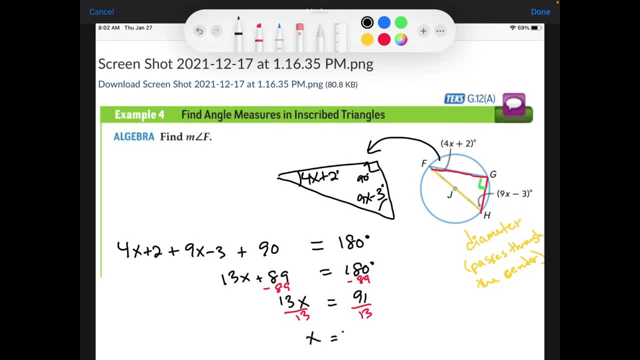 Dividing both sides by 13 would give me X is equal to 7.. Now that is not the answer, because they want to find the measure of angle F. So the measure of angle F is equal to 4X plus 2.. 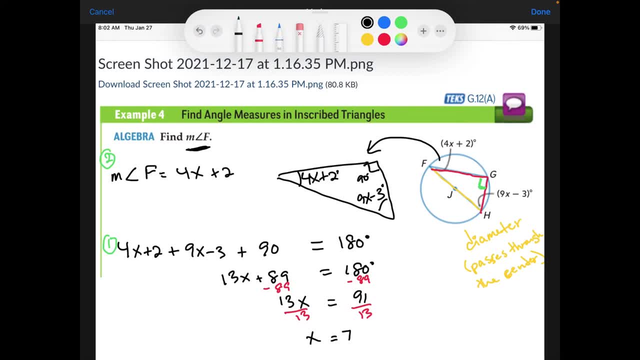 So I want to just remind you. this was step one and this is step two. We have to now plug in the information that we found here. X was 7.. Now that we have that in there, we can simplify this: 4 times: 7 plus 2 is going to give me 30.. 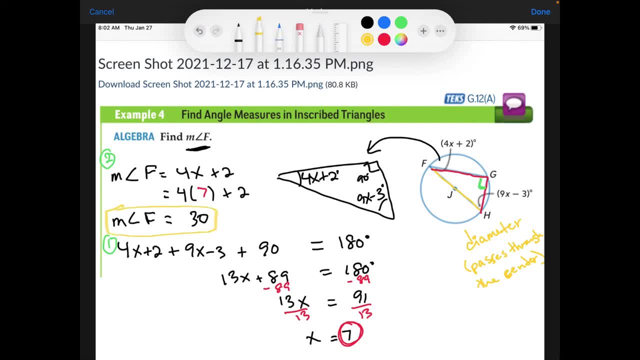 So this is now the measure of angle F. Like I always say, you know, try to find the positive in math. It is difficult and hard, but just like working out, sometimes you got to get it to burn before you see the growth. So once again, have fun with it, stay positive and I'll see you in the next video. 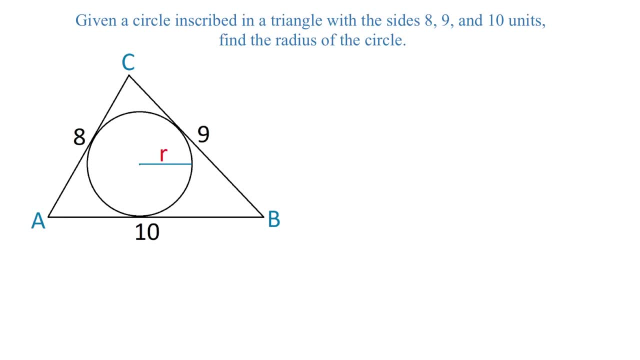 Given a circle inscribed in a triangle, with the sides of 8,, 9 and 10 units. find the radius of the circle. To find the radius of this circle, we will start with finding the area of the triangle. Then, once we have the area of the triangle, you will see how we can form an equation that will give us the radius of the circle. 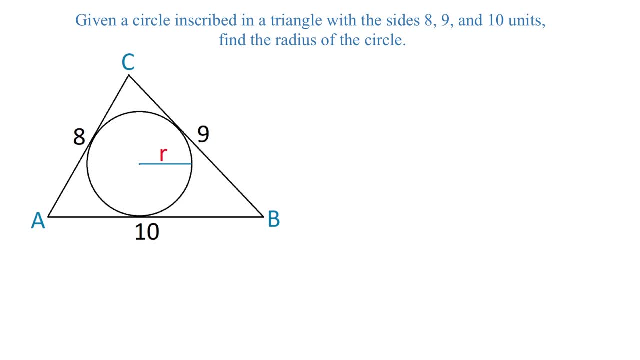 In this triangle because we are given all three sides. to find the area, we will use the Heron's formula. This formula has two parts and in part 1, we are finding half of the perimeter of the triangle with the sides A, B and C. 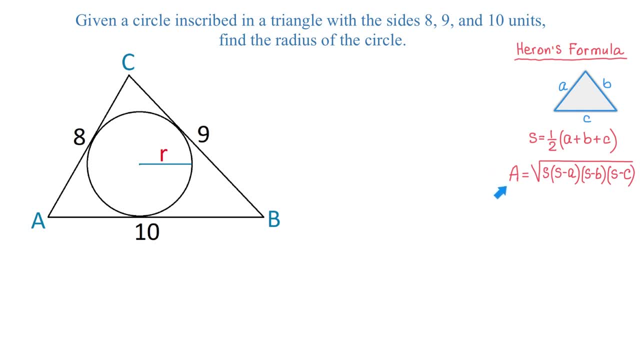 Once we find number S, we use it in the second part, where we find the area of this triangle. This formula is square root of S, times S minus C, S minus A, times S minus B and times S minus C. Now in our problem, S equals 1 half times 8 plus 9 and plus 10.. 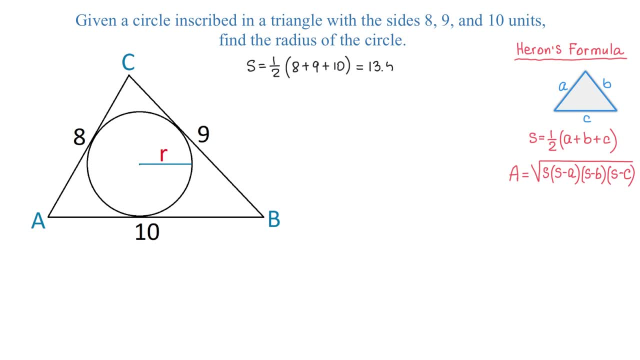 All this equals 13.5.. Now, in the second part, the area equals the square root of 13.5 times 13.5 minus C. Now, in the second part, the area equals the square root of 13.5 times 13.5 minus C. 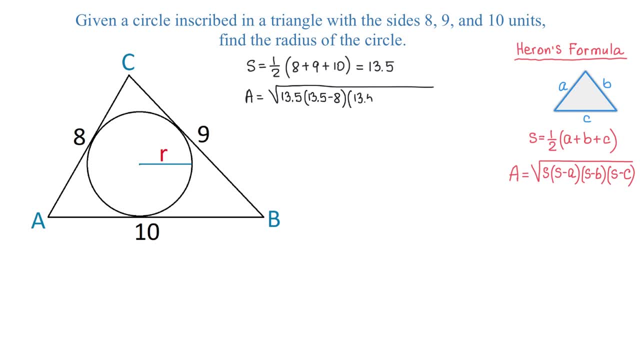 S minus A times 13.5 minus 9 and times 13.5 minus 10.. Now in the third part, the area equals S minus A times 13.5 minus C, S minus A times 13.5 minus 9 and times 13.5 minus C.